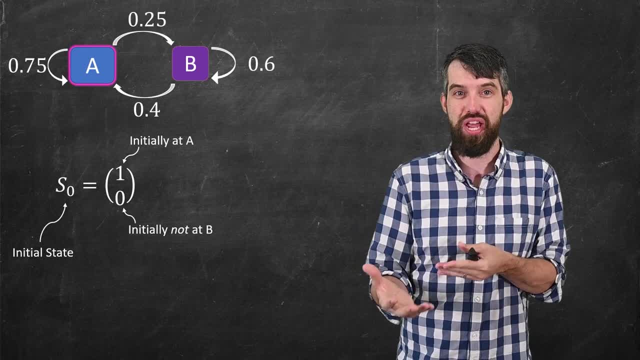 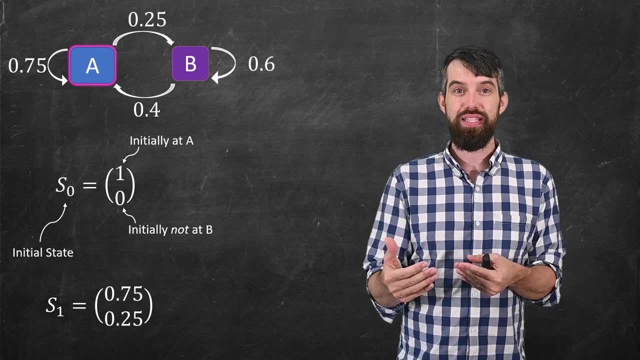 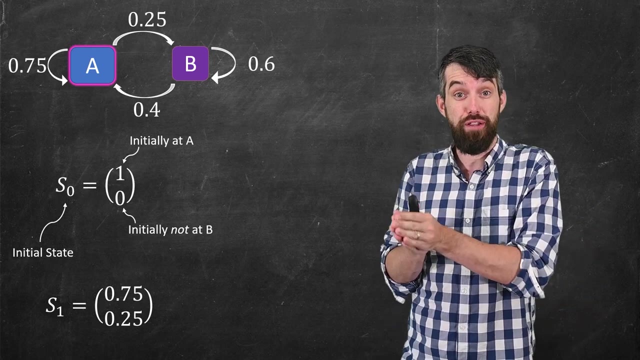 the system. Indeed, I sort of highlighted it in pink in my transition diagram just to illustrate. I'm starting at state A. Okay, Then I want to go to S1.. S1 is the state after one iteration. That is, if I start at my S0,, my initial state, and go one iteration into the future, I am then at S1,. 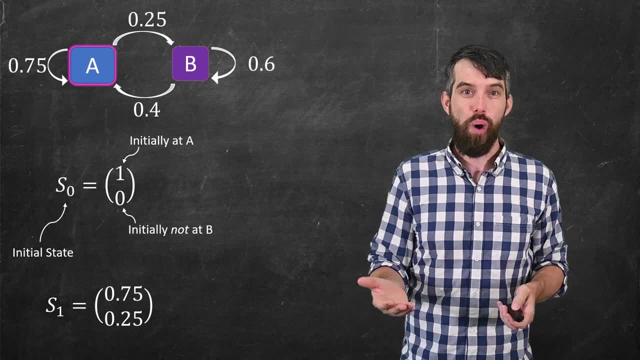 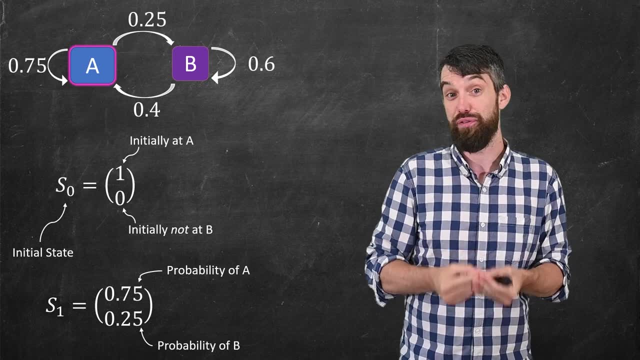 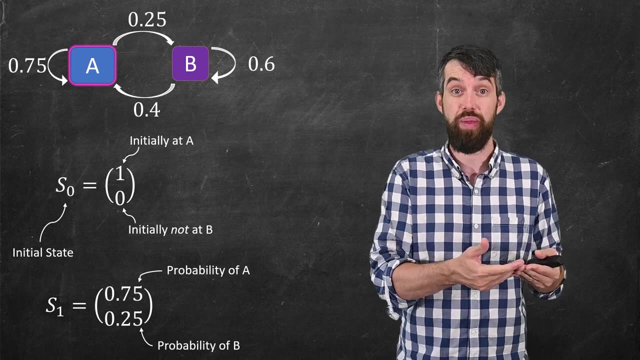 the state after one iteration, And likewise the 0.75 and the 0.25, the top number is still referred to as the state B, And so the 0.75 and the S1 is referring to the fact that there's a 75% chance of. 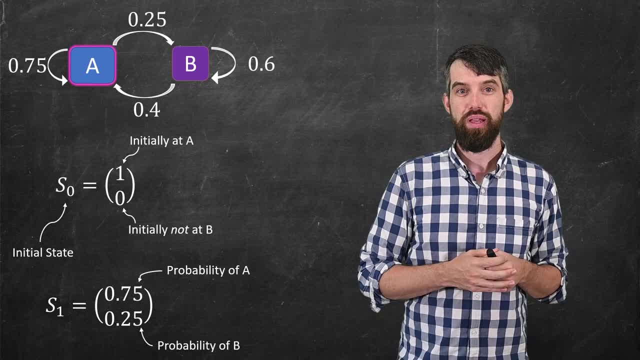 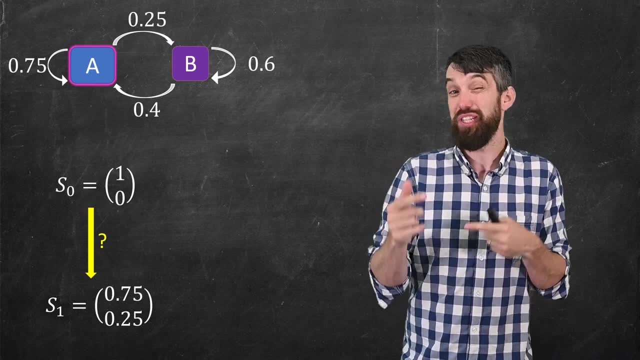 it being back in state A after one iteration. So then the question becomes: how can I manipulate to go from the S0 to the S1? I mean, in this case we were able to sort of figure out what the S1 was. 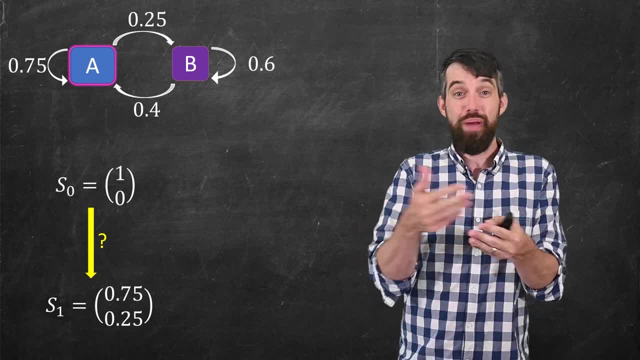 just by looking at the diagram, But I can then follow up on this. Well, how do I go from S1 to S2, the state after two iterations, Or S2 to S100? Is there a process that I can use to do that Well? 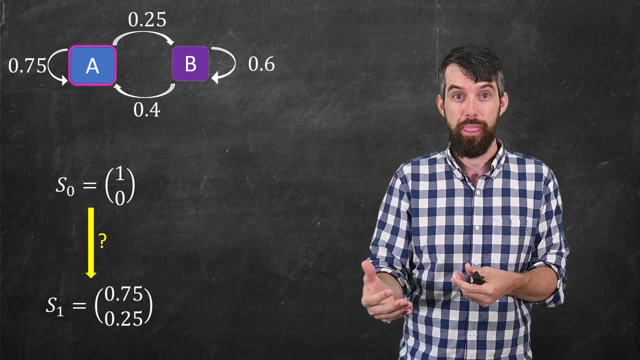 S2 to S100?. Is there a process that I can use to do that? Well, S2 to S100?. Is there a process that I can use to do that? Well, S2 to S100?. Is there a process that allows me to do those types of manipulations efficiently? 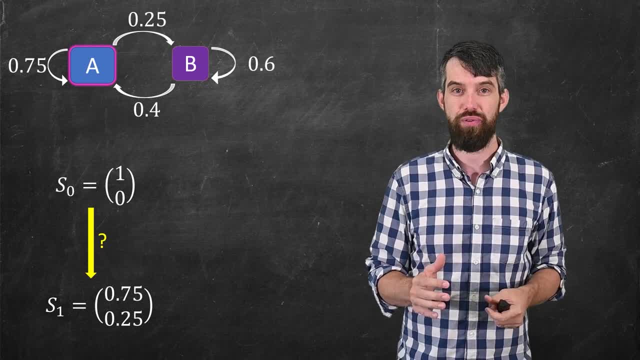 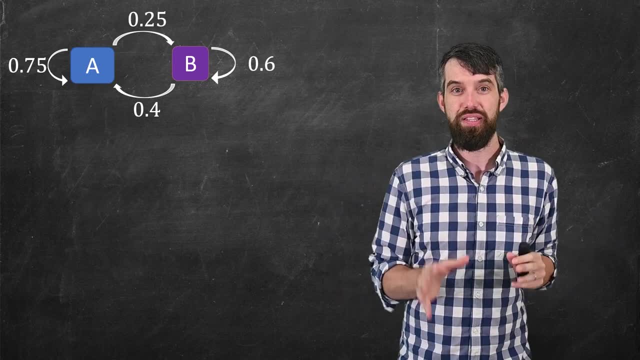 And indeed the answer is yes, there is, And we're going to use the notion of a matrix. How this works is: let's consider the transition diagram. There are four numbers, So let me just forget the rest of the diagram for a moment and just pull those four numbers. 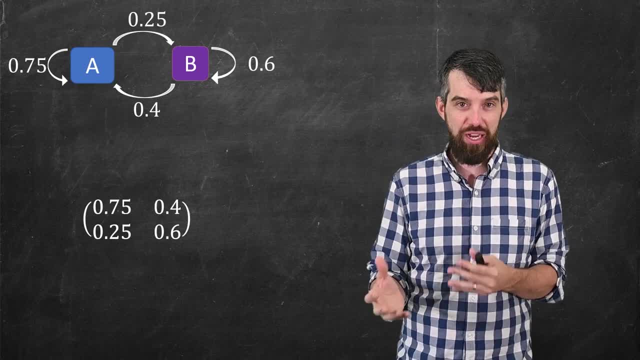 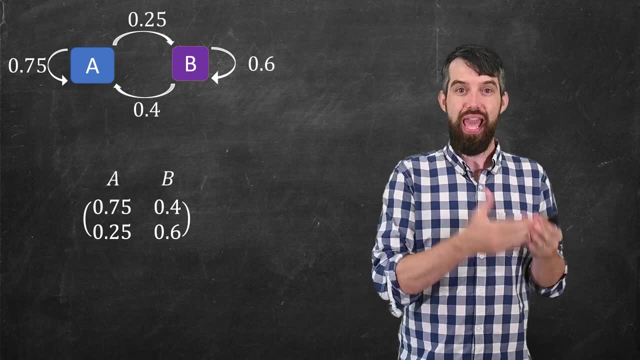 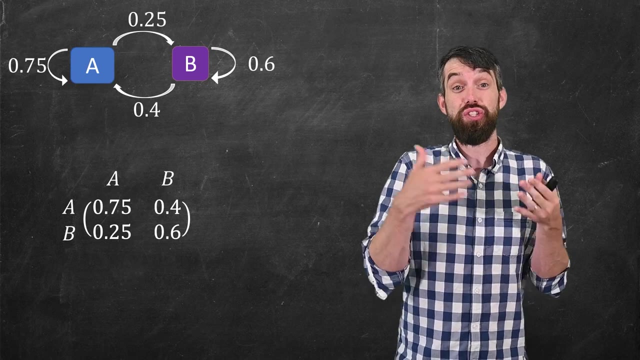 together. This is going to be called a matrix, an array of different numbers. The way I think about this is: I imagine that my columns are denoted with an A and a B, and I imagine that my rows are denoted with an A and a B, So something like the 0.75 represents if I start in state A, I will end. 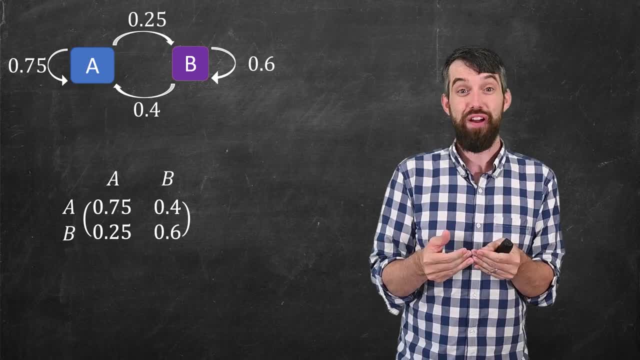 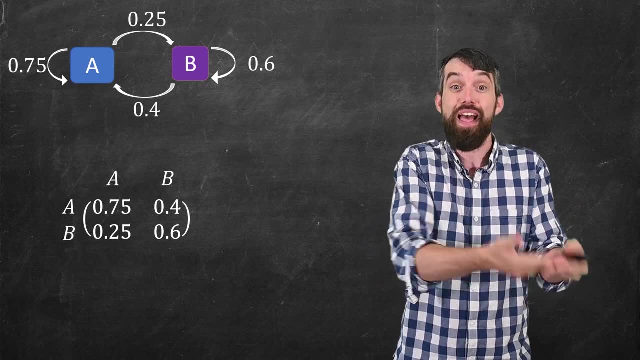 up in state A. Something like the 0.4 says: if I start in state B, it's in the second column, so if I start in state B, then I will end up in state A. That's what the 0.4 represents. This type of 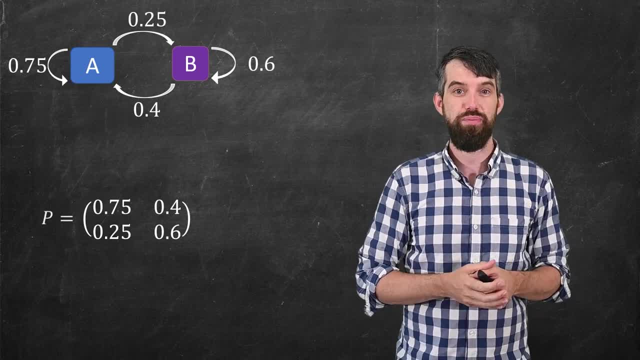 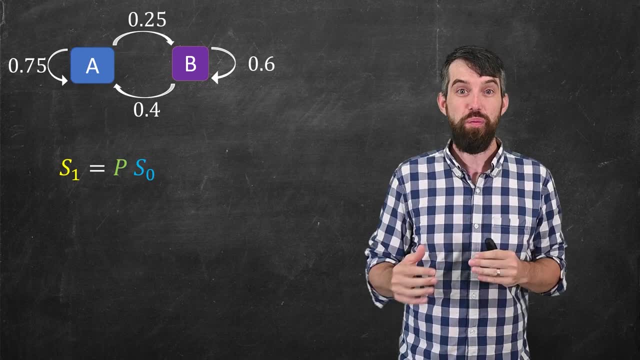 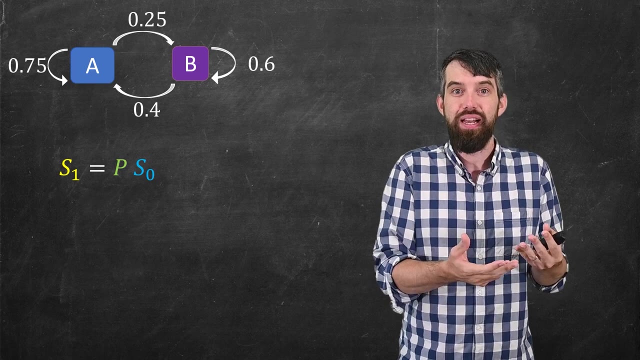 matrix is called a transition matrix and we often just write it as P for the transition matrix. Now here is the logic of matrix algebra. The formula to go from S0 to S1 is just multiplying by this matrix P. In other words, S1 is P times S0. And if I want to write that out with the actual information in: 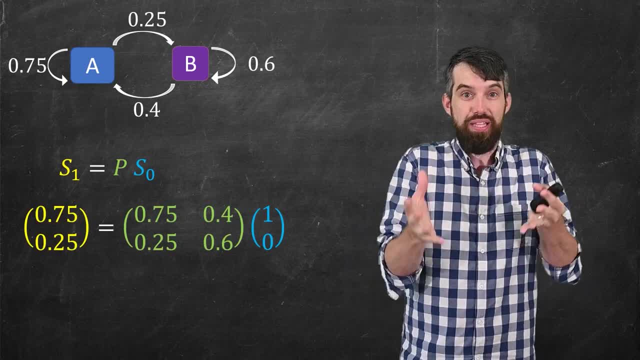 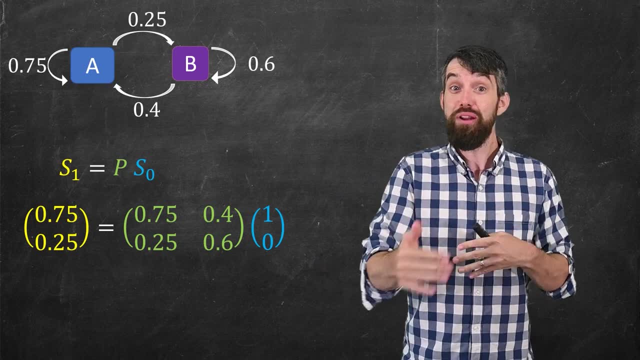 this case, the S1 was the 0.75, 0.25, the P was that matrix and the S0 was the 1, 0. This is matrix vector multiplication. Now, if you don't know what matrix vector multiplication is, that's. 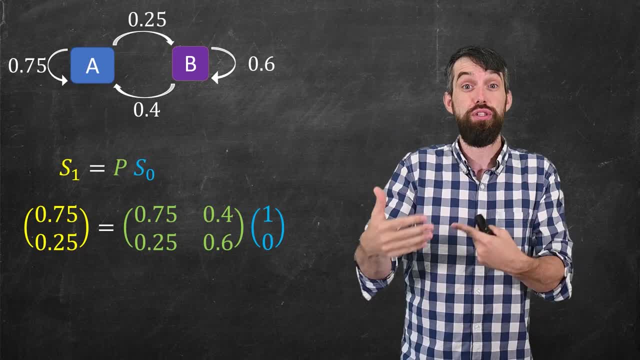 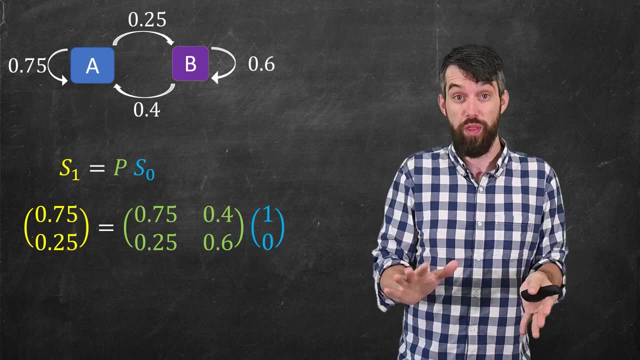 totally fine. So I have a video for you that introduces matrix vector multiplication. It has nothing to do with Markov chain, specifically because this little piece of algebra is useful all over the place And I would encourage you to check that video out and make. 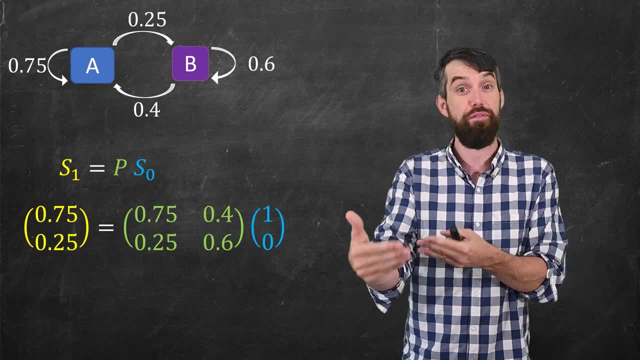 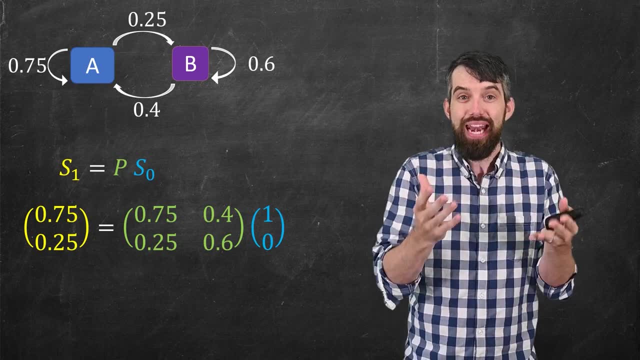 sure you're comfortable doing matrix vector multiplication. I'm just going to assume that for the rest of this video. Nevertheless, for the purpose of this particular video, all that's worth noting is that when you do this multiplication on the right, you get exactly that vector that. 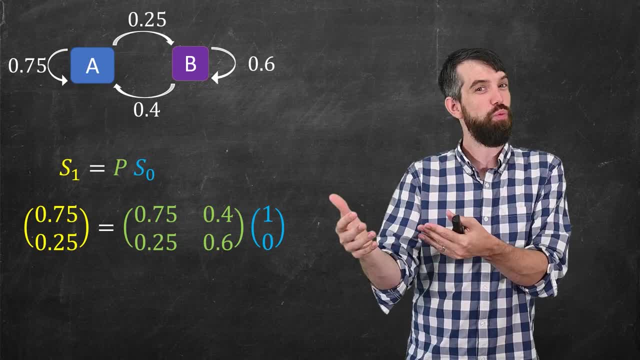 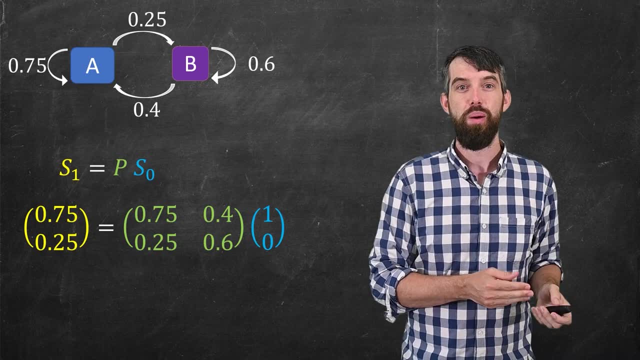 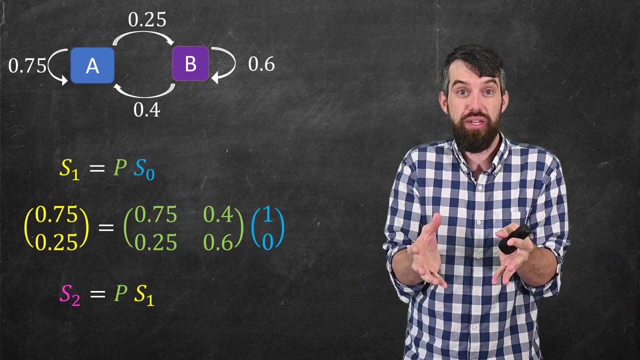 we predicted on the left. Now, thus far we haven't really gotten a big improvement, because you were capable of coming up with the S1 just by looking at the diagram. We didn't mean to do all that. But what about going towards S2?? The second state is again. just take that transition matrix. 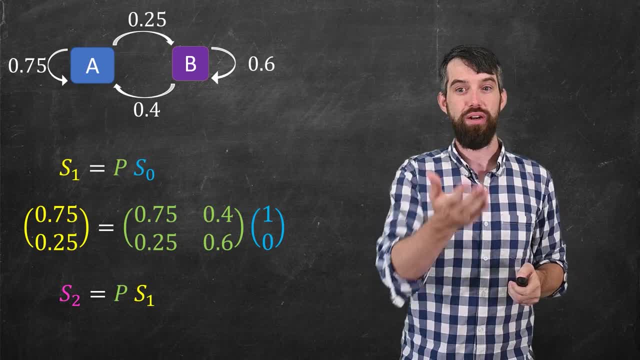 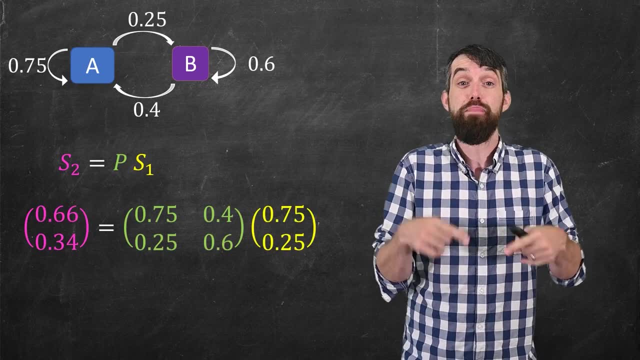 and multiply it now to the S1.. In other words, I can go and take a look at this. This is going to be a new multiplication: that same transition matrix but multiplied by 0.75, 0.25.. And if you do that, 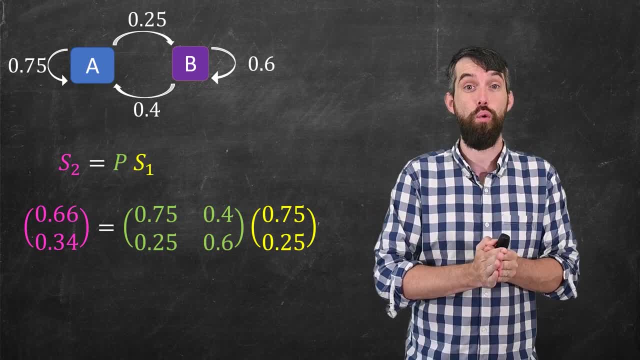 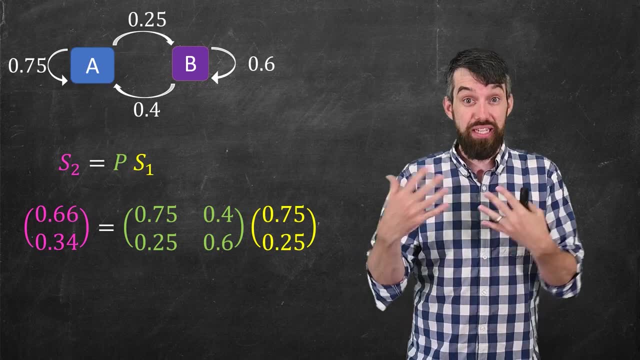 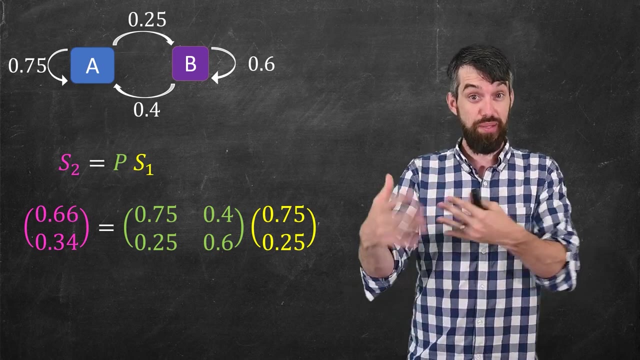 matrix vector multiplication, you get 0.66, 0.34 for the S2.. Now I want to note that in the first video on Markov processes, we actually did this computation via a tree diagram and I showed how to justify it. And so right now I really just want to note that, using this matrix method, 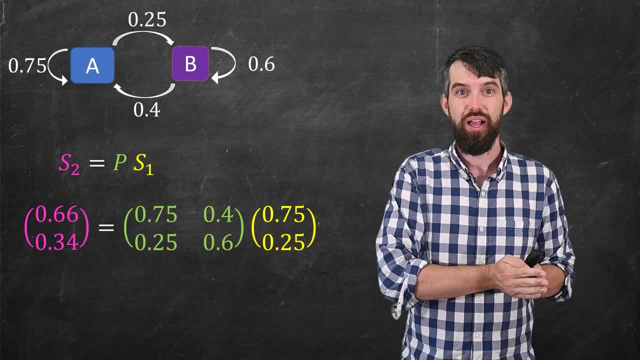 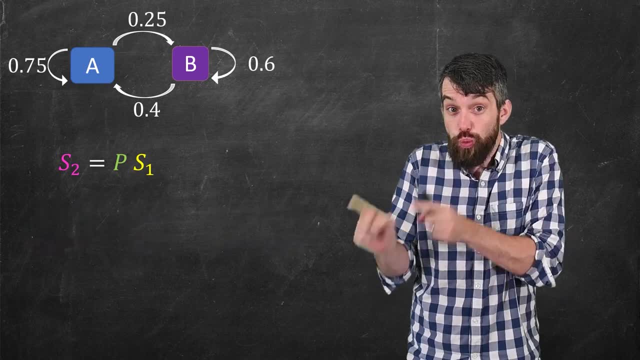 gives us the same answer that we've done in the past, But now it generalizes. What have I just done? If I just look at this, S2 is P times S1.. S1 was P times S0.. So, in other words, what this is. 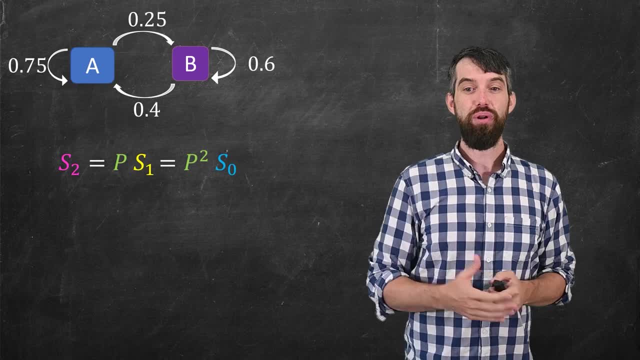 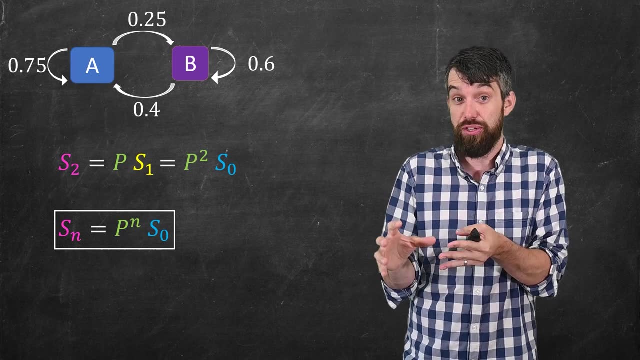 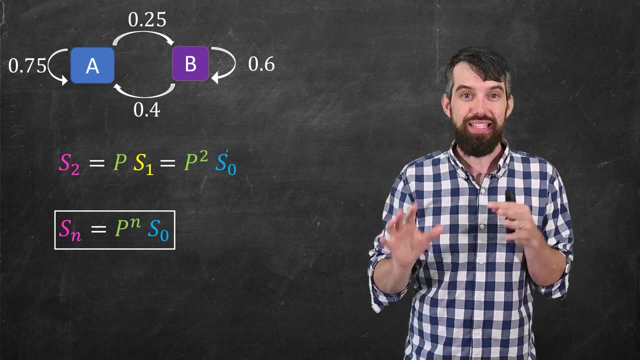 is P squared times S0.. And, in general, if I wanted to figure out what the nth state of my Markov processes would be, it would be just start at the S0, start at the initial state and then multiply by n transition matrices P to the n. And this is my final answer for how I